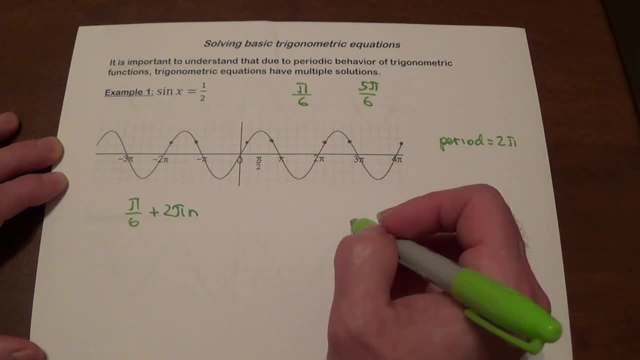 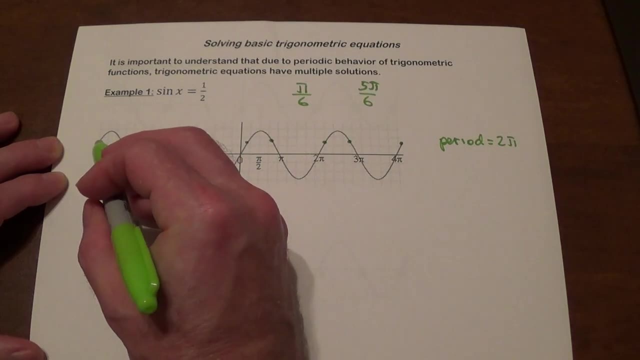 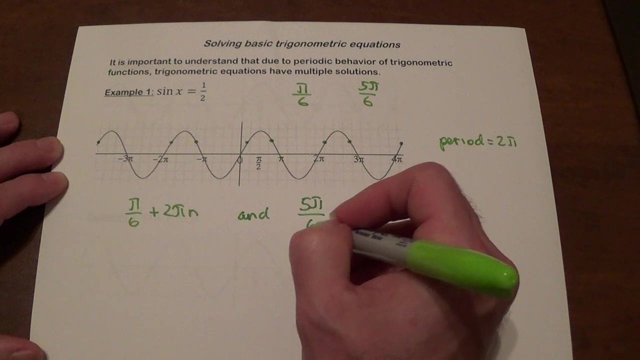 So, we add 2 pi n, where n is an integer, that's going to give you a set of solutions, it's going to be this point, that point, that point, that point, another point here, and also, it's going to be 5 pi over 6 plus 2 pi n. 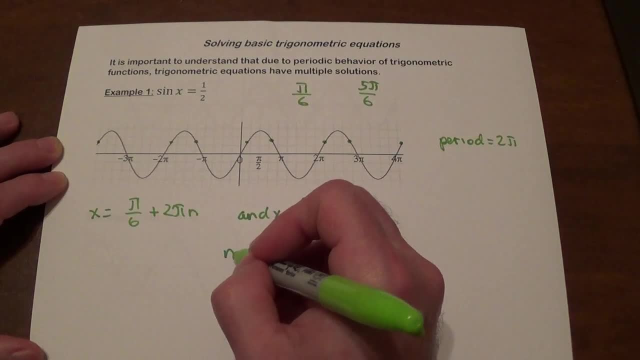 So, it's x equals x equals n is an integer. Okay? Moving on. 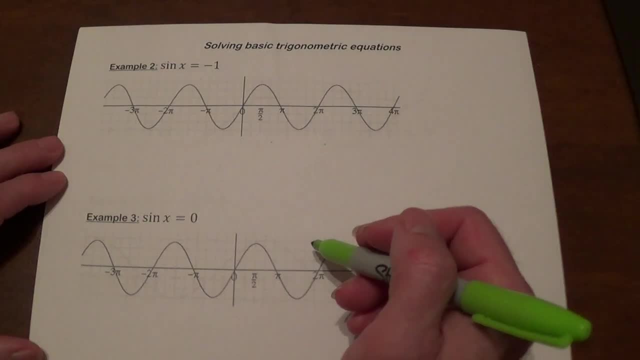 Sine x equals negative 1, where the sine reached the value of negative 1. There's one point here at 3 pi over 2, then it will repeat itself again every 2 pi. 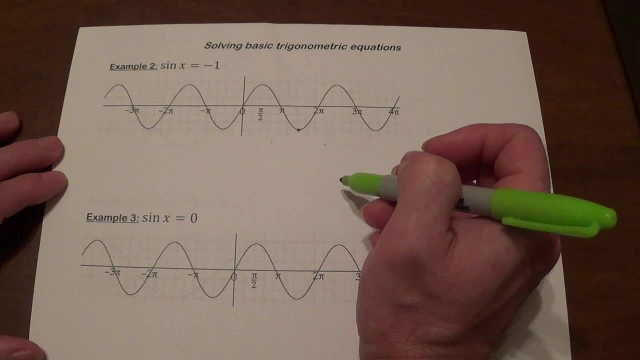 Because it reaches one of the extreme values, because it's the lowest value that time can attain, then it's going to be only 1. 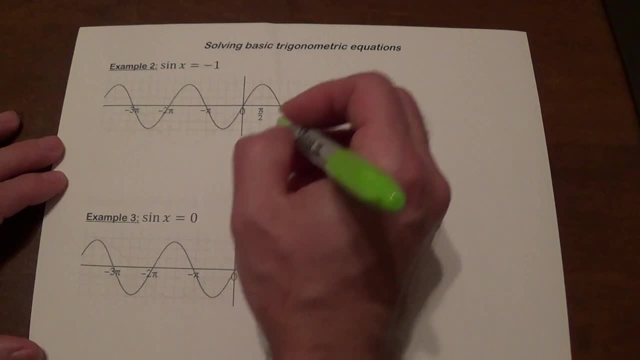 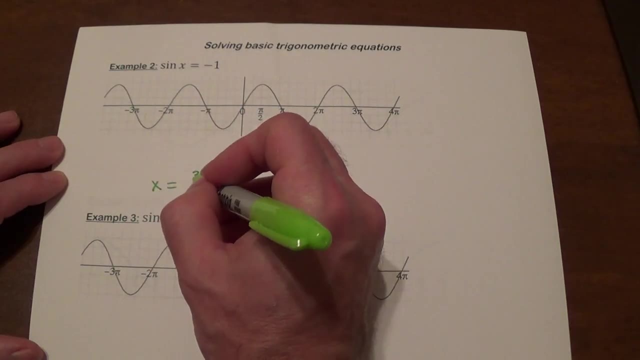 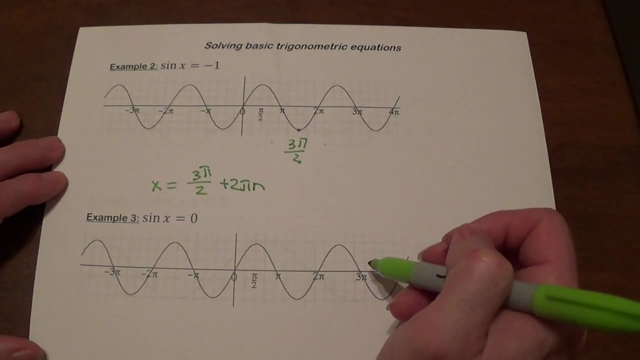 So, it's going to be a point like that, but it's going to repeat every period. So, we're going to have, this is 3 pi over 2, and our solution is going to be x equals 3 pi over 2 plus 2 pi n, where n is an integer again, and it's going to give us that. 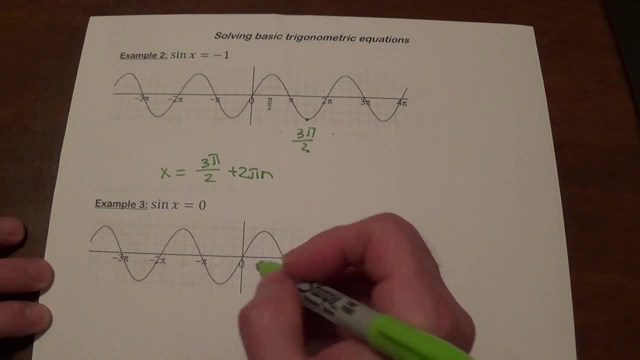 Sine x equals 0. Well, when sine x equals 0, that's going to happen at 0, but then it happens again at pi, it happens again at 2 pi and 3 pi. So, that's, that one value is going to be attained at each one of these points, and it's also going to repeat itself every pi, even though the period of sine function is 2 pi, these values are going to repeat every pi. 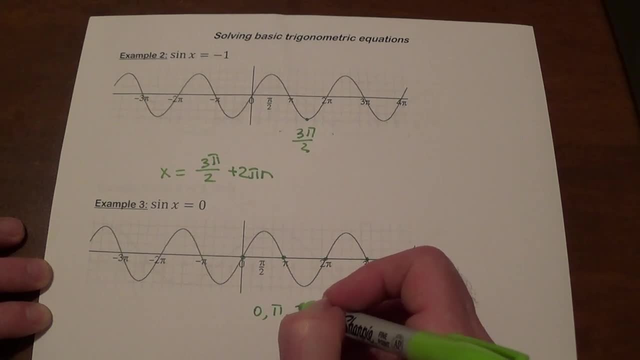 So, if you write 0, then you have pi, then you have 2 pi, I have negative pi, all that's going to fall under this, it's going to be pi n, where n is an integer. 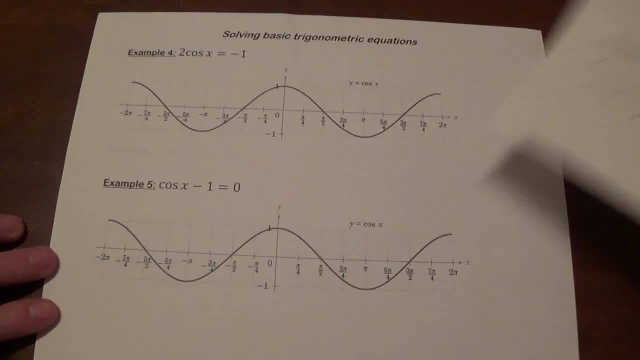 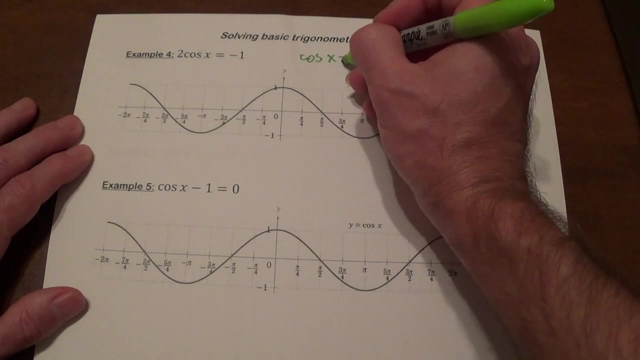 Okay? 2 cosine x equals negative 1. So, the first thing we need to do is leave cosine by itself. So, it's cosine x equals negative 1 half, we divide both sides by 2, and now we can go ahead 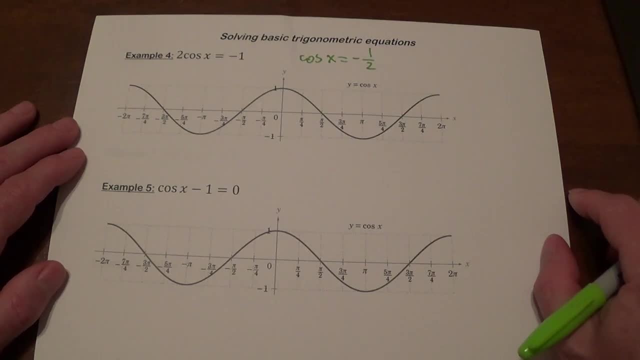 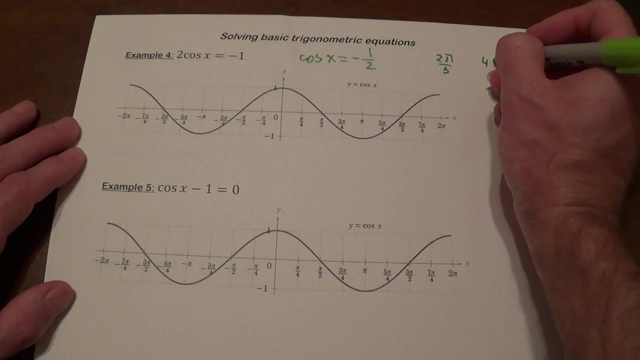 and do it, where is the value of cosine going to equal negative 1 half? It's going to happen at 2 pi over 3, and it's also going to happen at 4 pi over 3. 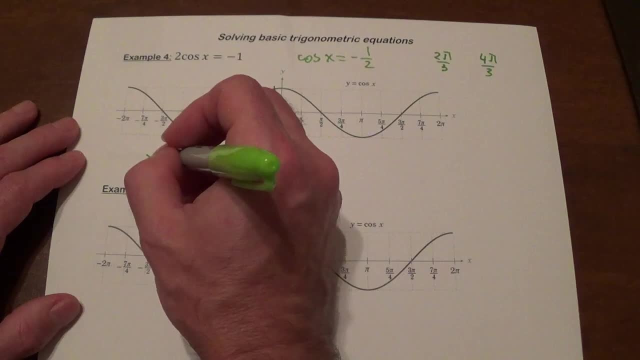 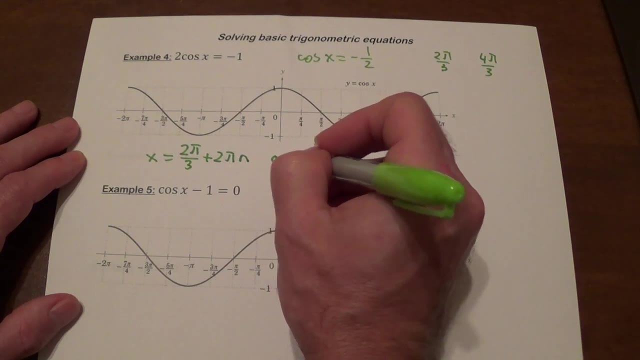 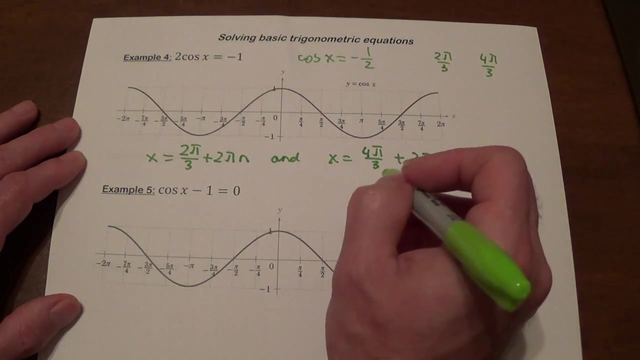 So, we take each one of them. Okay? And we add 2 pi to it, so 2 pi over 3 plus 2 pi n, and x equals 4 pi over 3 plus 2 pi n. 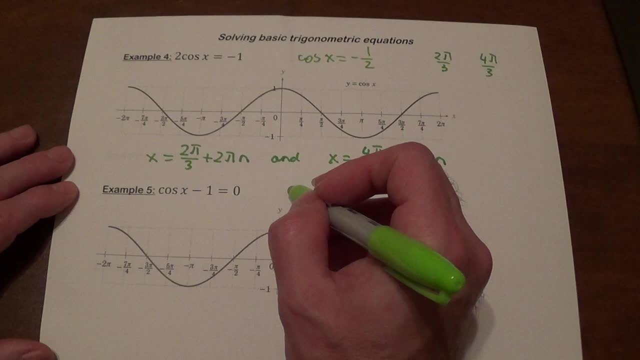 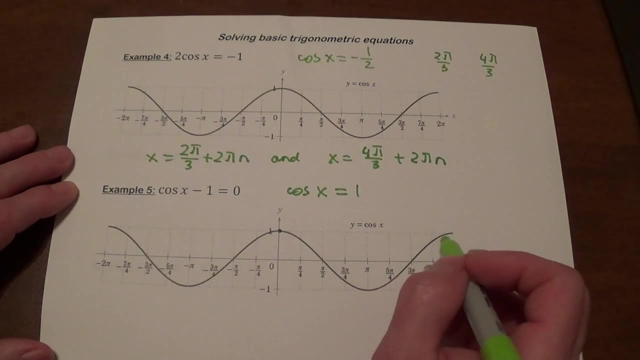 Cosine x minus 1 equals 0, first let's rewrite that, cosine x equals 1, where does that happen? It happens at this point. And then at each point over here. 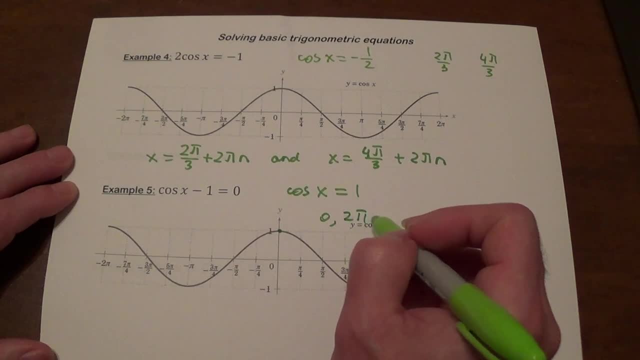 So, it's going to happen at 0, it's going to happen at 2 pi, it's going to happen at 4 pi, it's going to happen at negative 2 pi. 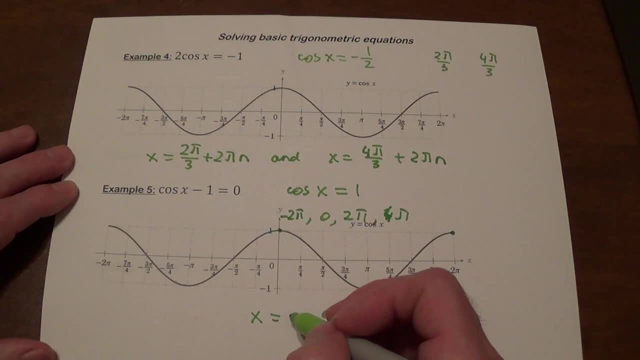 So, these can all be described as 2 pi n. Okay? 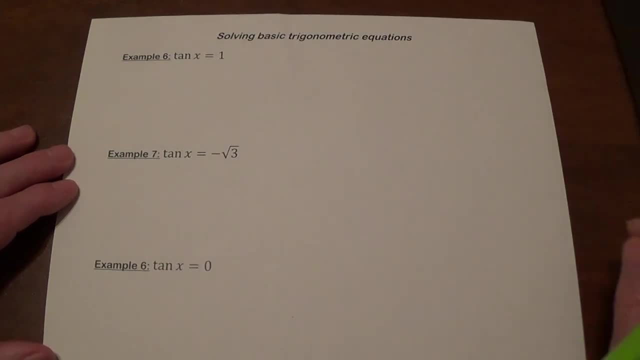 Example 6, tangent. So, remember tangent, the period of tangent, is pi, and also tangent, the graph of tangent is the one that goes like that and what happens is 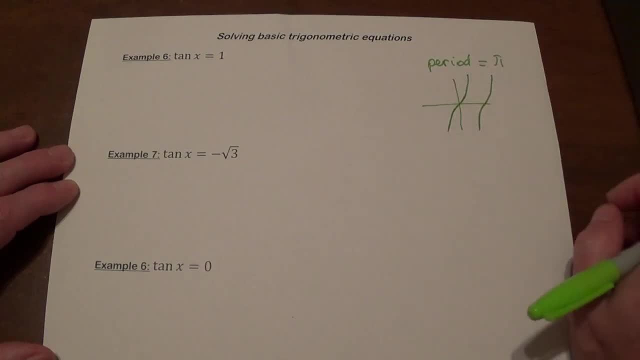 it's not going to have up and down like sine and cosine do, so it's a little bit easier in the way. 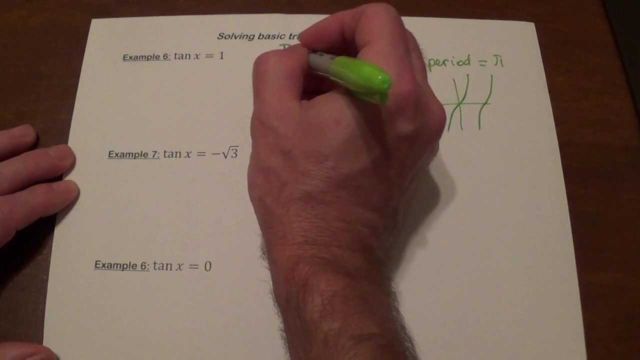 Where is tangent going to equal 1? Tangent equals 1 on pi over 4, it's going to repeat every pi, so the answer here is going to be x equals pi. 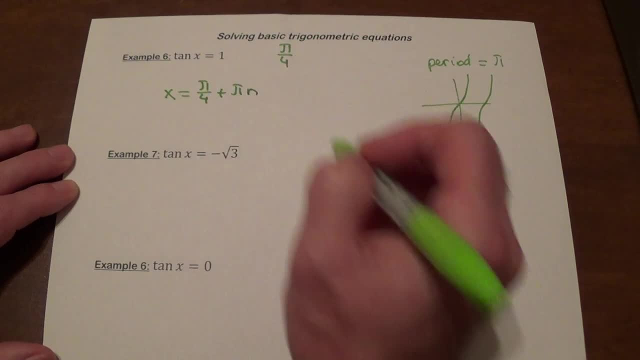 Pi over 4 plus pi n. 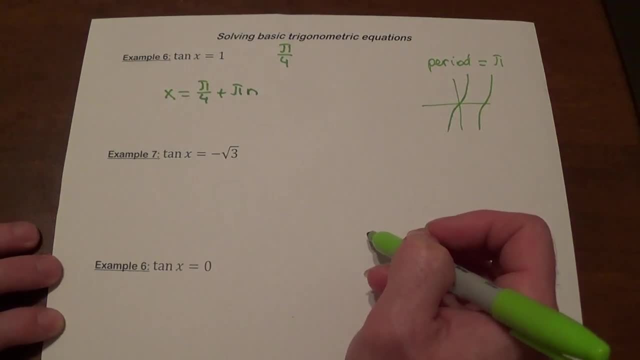 Tangent x equals negative square root of 3, where is tangent going to be negative square root of 3? 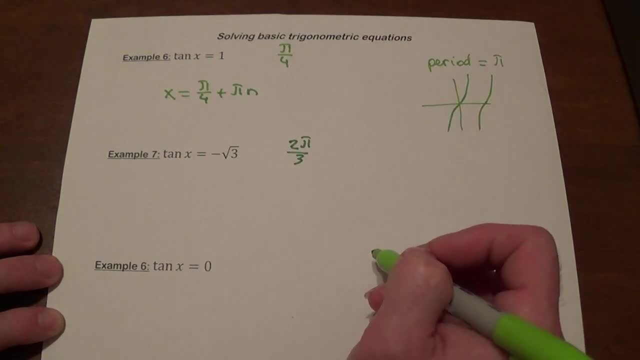 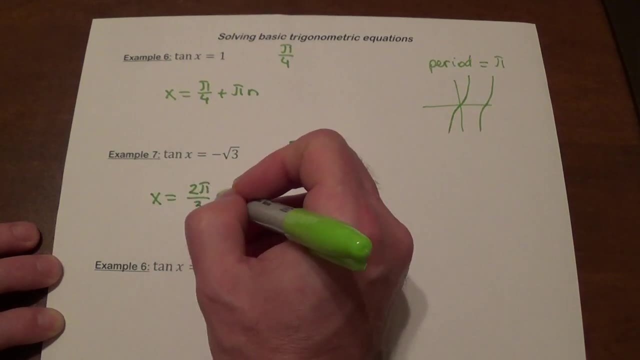 That's going to happen at 2 pi over 3. And it's going to repeat every pi, so the value of x here is going to be 2 pi over 3 plus pi n. Okay? 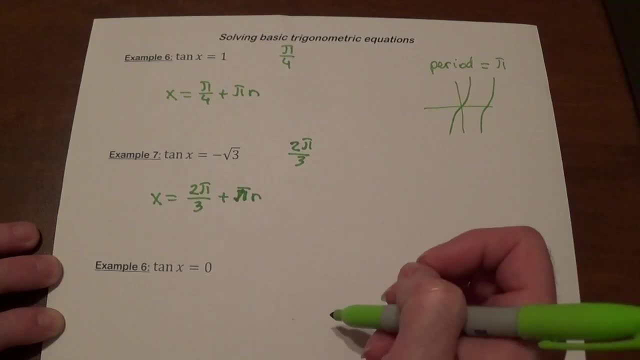 And tangent equals 0, where is tangent 0? At 0, and it's going to repeat every pi, so here the answer is going to be x equals pi n. Okay? 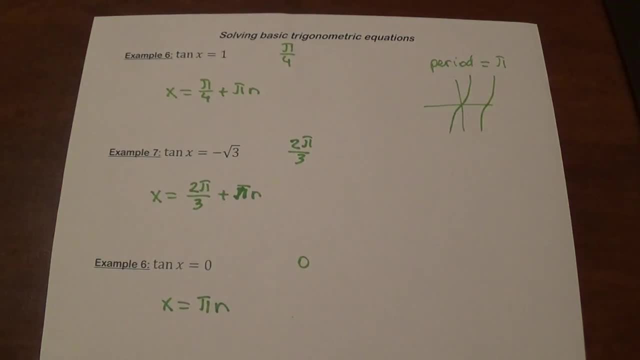 We'll do another video where it's going to go into more depth with some problems that you may run into, but that's just the introduction. Okay. Hope this was helpful.